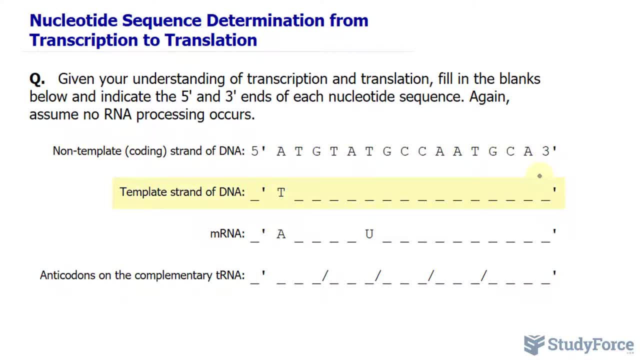 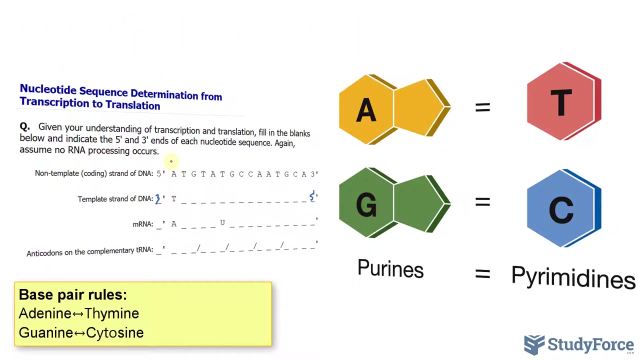 What is used is the template strand of the DNA. So if this nucleotide sequence is going from five prime to three prime, then the template strand will be three prime to five prime. It's always anti-parallel, So A base pairs with T and vice versa, while G base pairs with C. A is adenine, T is thymine. 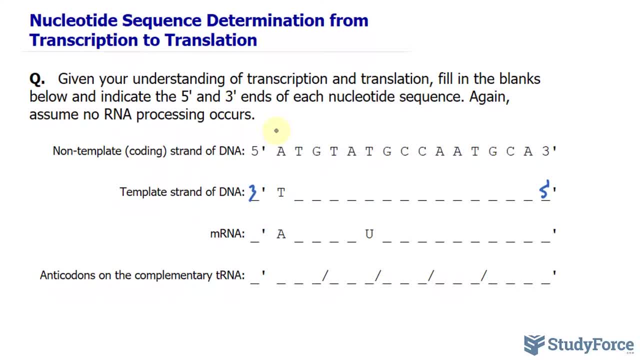 G is guanine and C is cytosine. That being said, if that is T, then here we should have A, And if that's G, we should have C, T, A, A, T and T base pairs again. 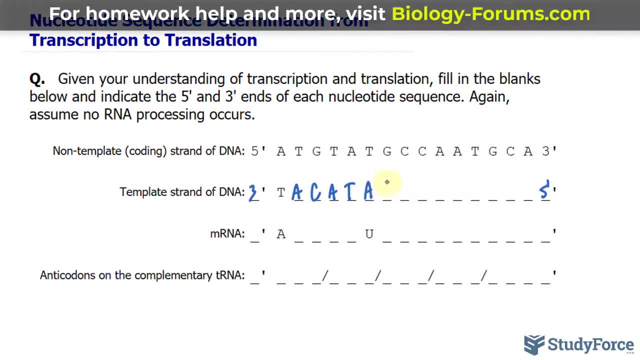 With A. The rest should look like this: C, G, G T, T, A, C, G T Moving forward. as mentioned, the template strand is what gets transcribed into mRNA. So, with that being said again, 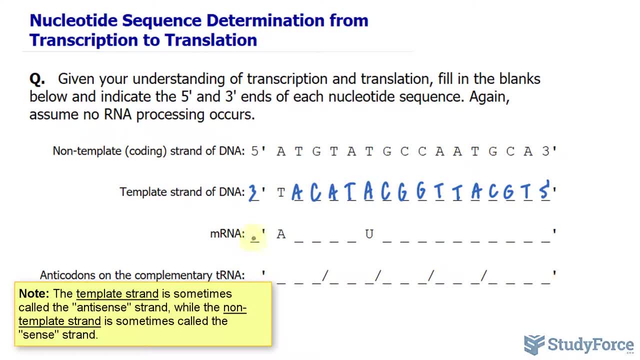 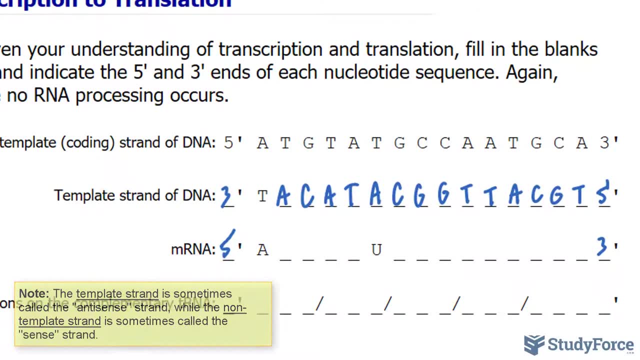 the mRNA should be running anti-parallel, So this should be five prime and that should be three prime. Now they've given you a few nucleotides already. They've said that T base pairs with A, but, unlike with DNA, the base pairing when it comes to mRNA is a little different. 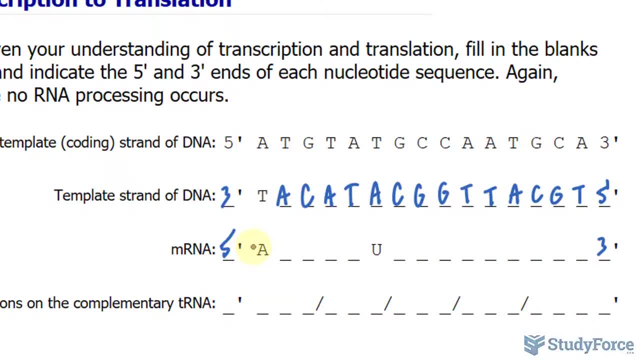 T base pairs with A, but A base pairs with U, which represents uracil. So wherever you see an A along this nucleotide strand, you should have a base pair with U. Now, that being said, mRNA or any form of RNA does not have Thymine. So if you ever have Thymine in the nucleotide, 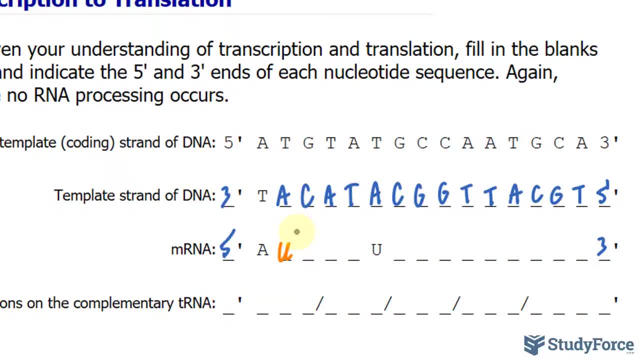 sequence of an RNA molecule, then it's incorrect. So C and G base pair, A base pairs again with U, T and A are both given and the rest should look like this, where we have G, C, C, A, C-A-A-U-G-C-A. 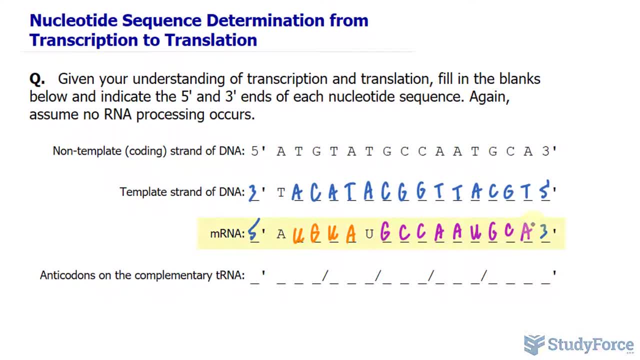 Notice how the mRNA sequence we just produced is identical to the coding strand of the DNA molecule, with the exception of U's replaced with T's. This is the reason the non-template strand is also called the coding strand, since it's the one that holds the code of the mRNA molecule. 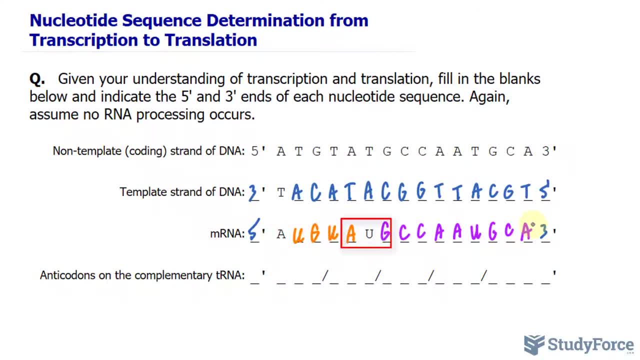 The mRNAs then read three nucleotide bases at a time after it forms a complex with the ribosomes. We call every three bases along the mRNA molecule a codon. This is why I included these slashes along the bottom row. tRNA molecules bring their respective amino acid. 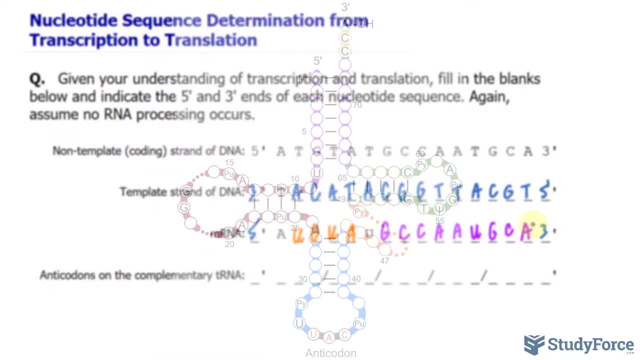 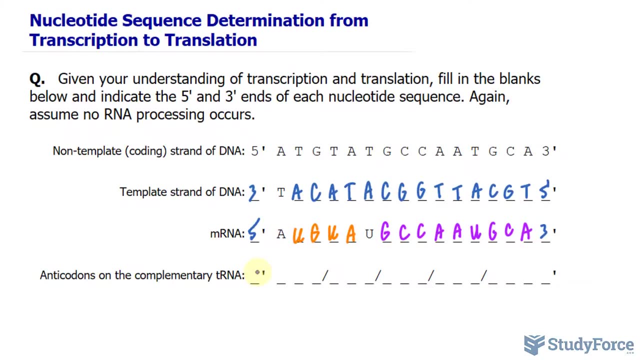 based on the sequence of the mRNA. Each tRNA molecule has an anticodon region that is complementary to the codon so that they hydrogen bond Again. this should be three prime and that should be five prime. Notice the same theme where you see five prime. 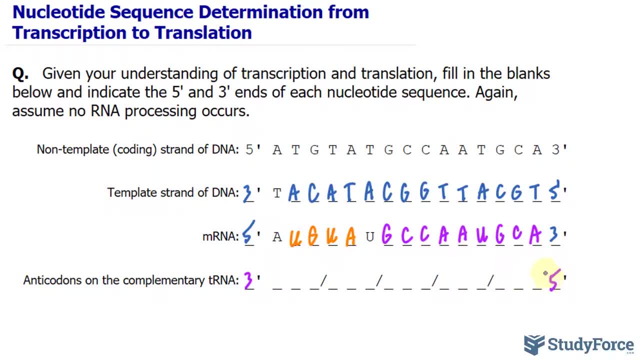 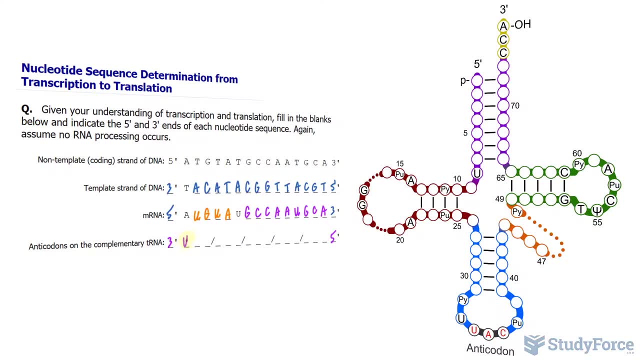 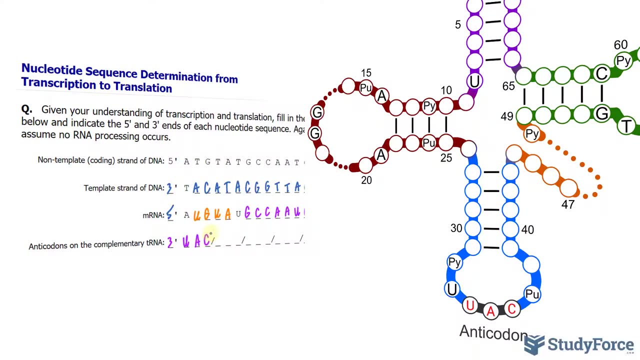 you should have three prime, and where you see three prime, you should have five prime. The anticodon will have a complementary sequence to this. So A will base pair with U, U base pairs with A and G base pairs with C. 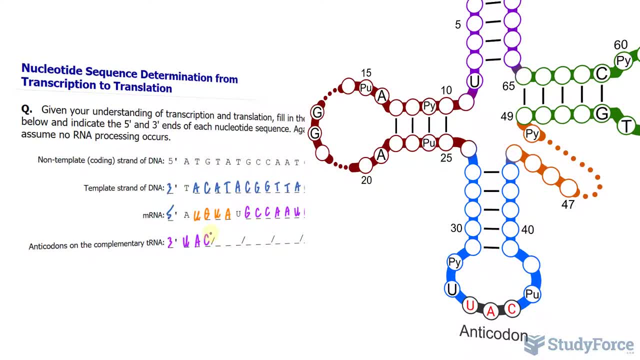 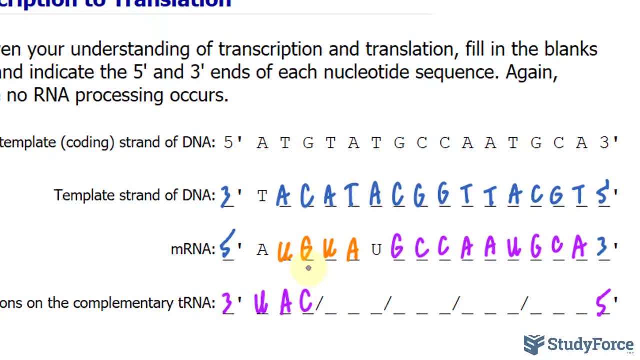 The tRNA molecule has to have this sequence and it's anticodon. The tRNA molecule has to have this anticodon region. Interestingly, when mRNA is AUG in its nucleotide sequence, methionine is the one that is connected to the tRNA. 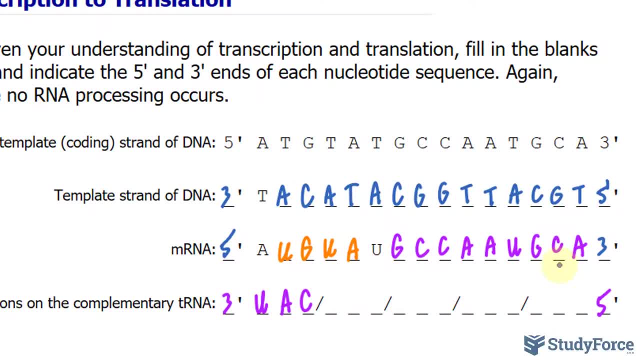 having this anticodon sequence. Of course, you can translate this using a codon chart like the one shown on your screen, but that's not the purpose of this question. U base pairs with A, A and U and we have the anticodon sequence A and U. 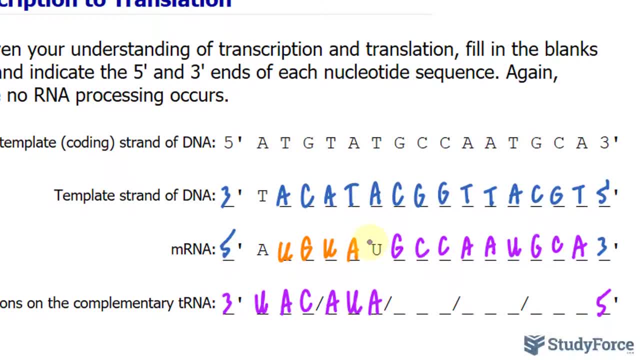 We have the anticodon sequence A, U, A for these three nucleotide sequences And the reason why they are separated with these colons is because those colons represent that every codon is three nucleotide base pairs: long G and C, G G. 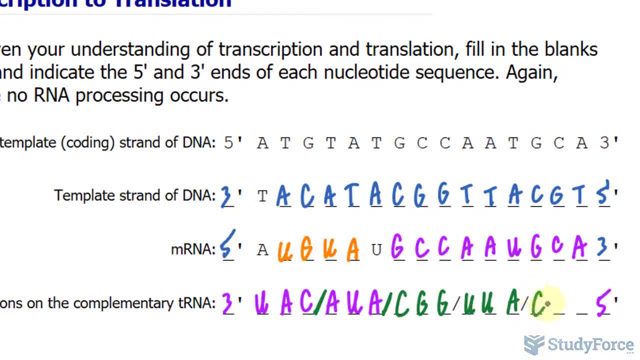 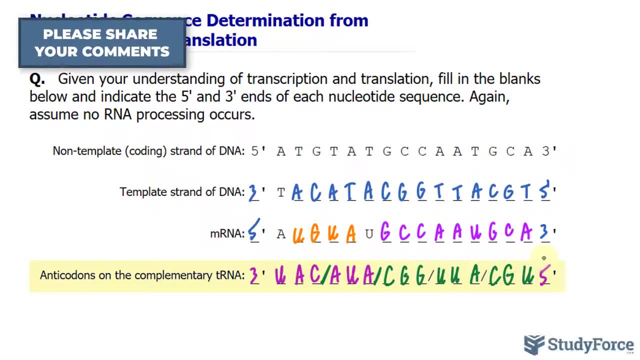 U, U, A, C, G, U. Notice how the anticodon is separated with these colons. The anticodons on the complementary tRNA strand are identical to the nucleotide sequence of the template strand of DNA, with the exception of T being replaced with U. 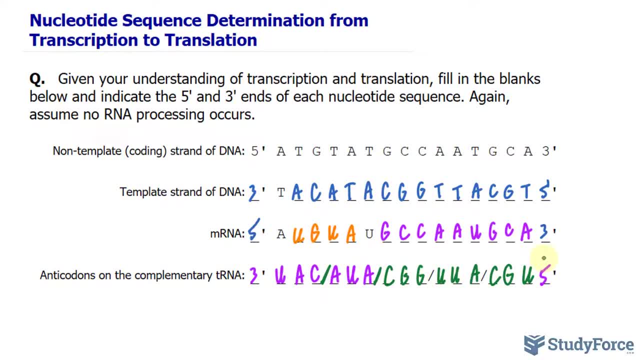 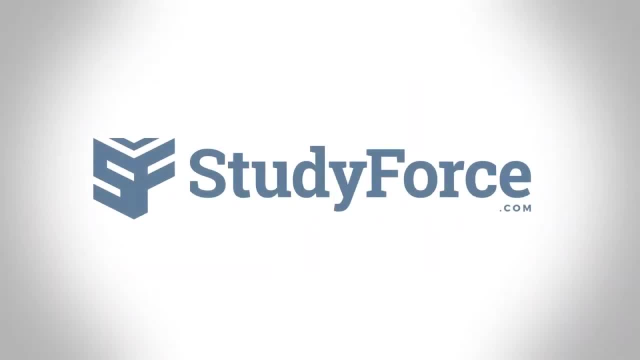 And there you have it. Now you know how to determine the nucleotide sequences for the template strand of DNA, the mRNA and tRNA anticodon. Thank you for watching.